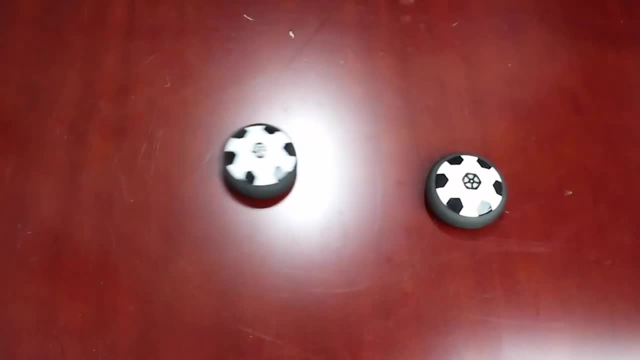 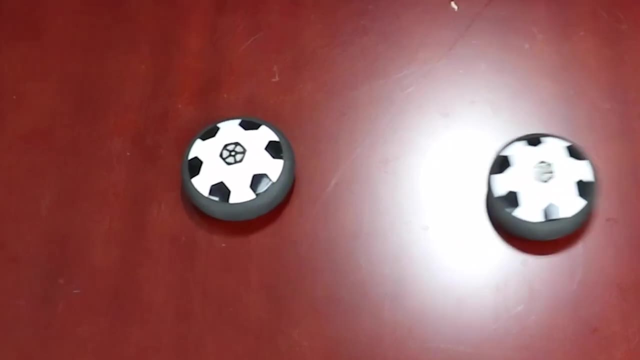 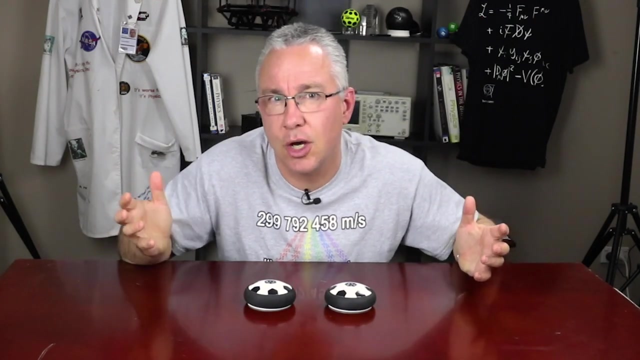 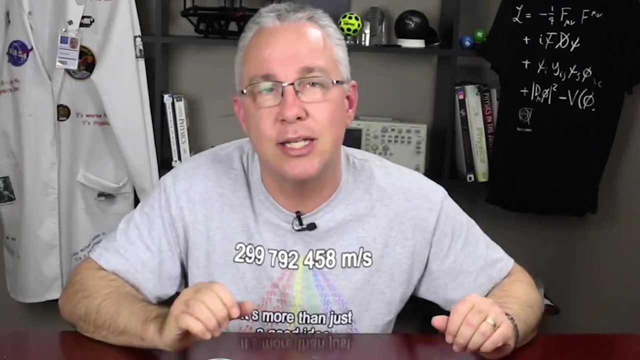 What makes this work? Well, clearly, this is a case of conservation of momentum. That is, this particle has momentum, it collides with this particle, gives it momentum and, as a result, they go off, and the total momentum before equals the total momentum afterwards. But what's the crucial? 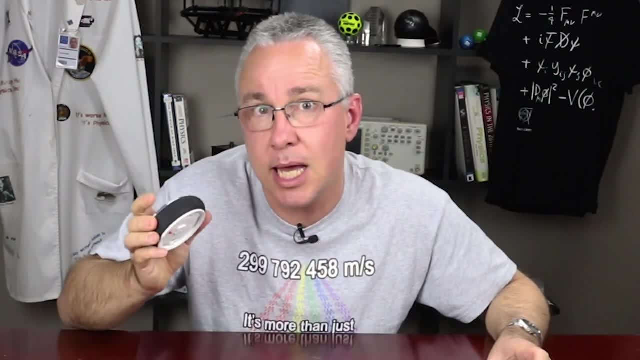 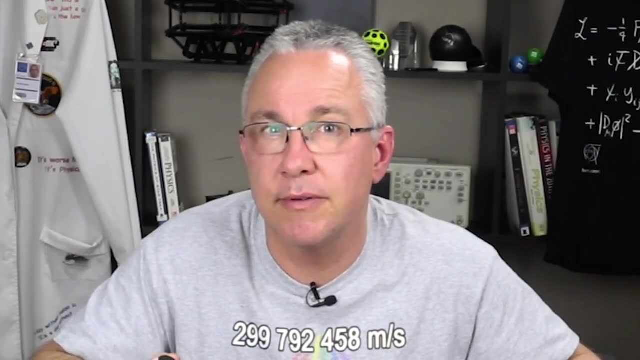 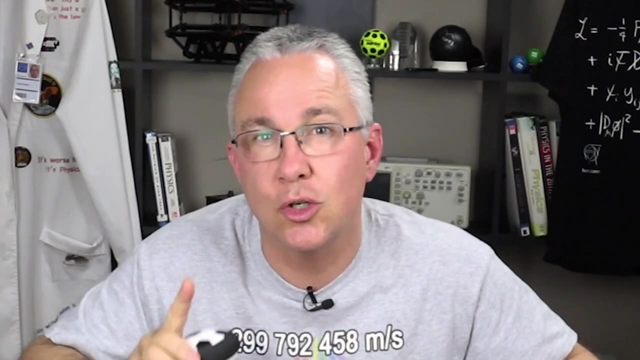 principle: for this to work, Well, this thing has to have mass. It has to have a certain amount of momentum to begin with for this to actually work. But what if I told you that I can make a conservation momentum work without having any mass to begin with? Well, that is the concept related to 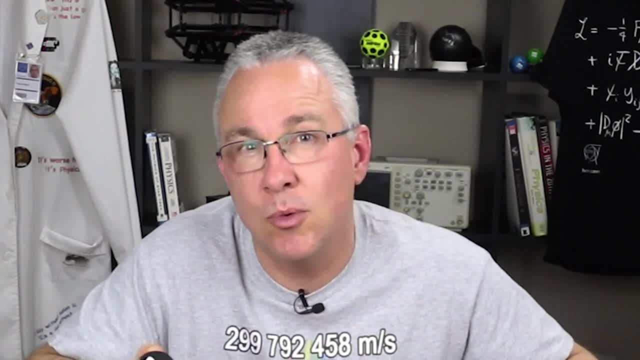 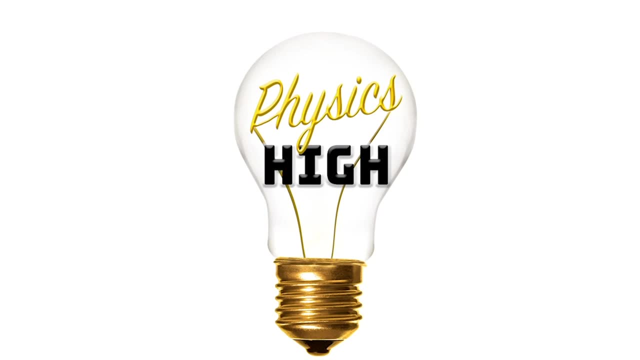 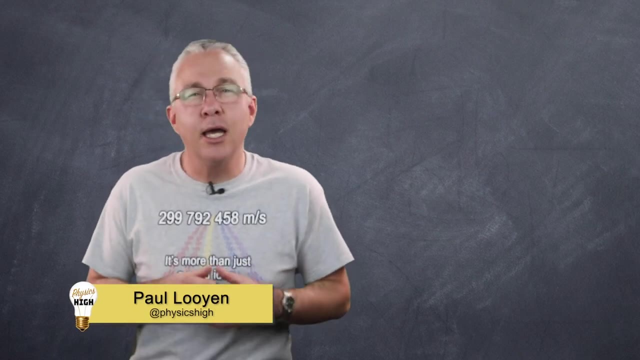 Compton Scattering or the Compton Effect. So to find out more about the Compton Scattering, stay tuned. Now, in 1905, in one of five papers that Einstein published that year, Einstein argued that light travelled in discrete packets. Now we call these photons now, but basically this explained what we. 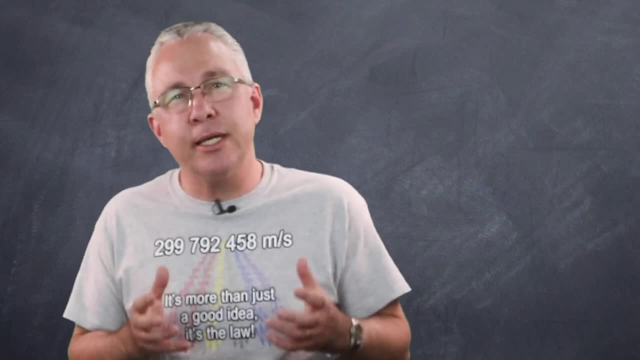 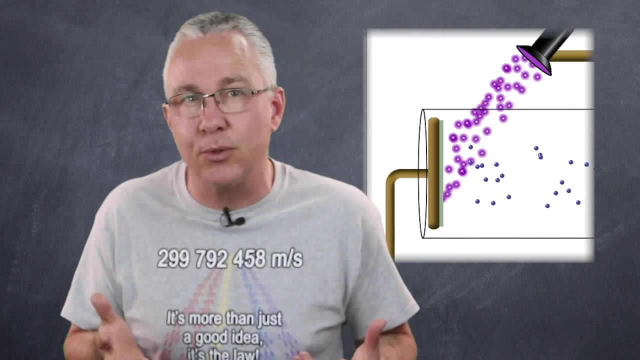 refer to now as the photoelectric effect, In other words the emission of electrons by shining light onto metals, could only be explained by treating light as a stream of particles. But really for the next 17 years there was really no consensus in the scientific community, In fact not all scientists. 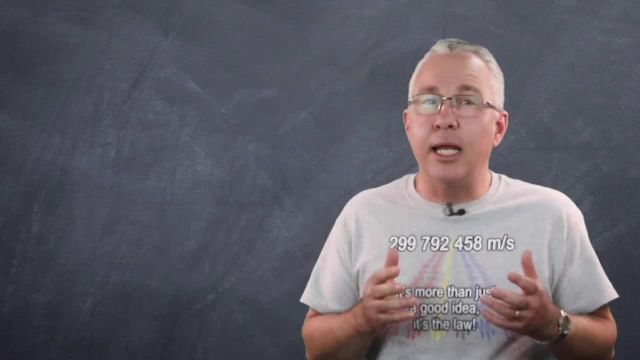 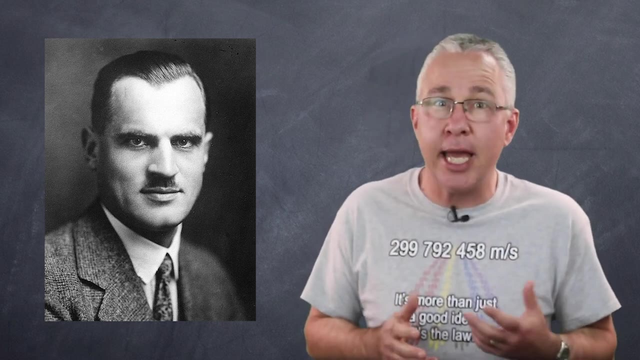 accepted the idea that light could travel like a particle. Now this is where Arthur Compton comes in. Soon after getting his PhD in 1916, Compton developed a keen interest in x-ray studies, especially in the use to study the arrangements of electrons and atoms in crystals. This then led to 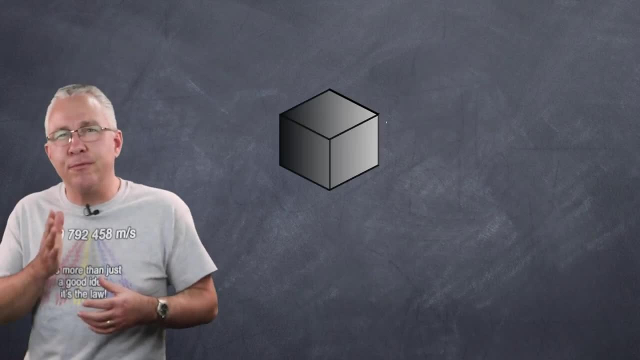 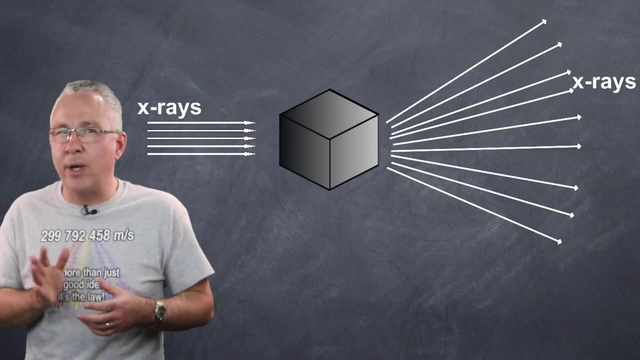 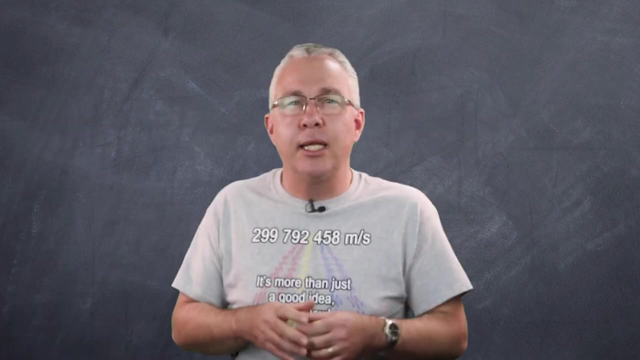 an interest in x-ray scattering. In essence, if we fire x-rays at crystals, then the x-rays are scattered off the crystal. But when Compton measured the wavelength of the scattered x-rays, they actually ended up like this: Now he basically set up a series of experiments to look at this more closely and then get a. 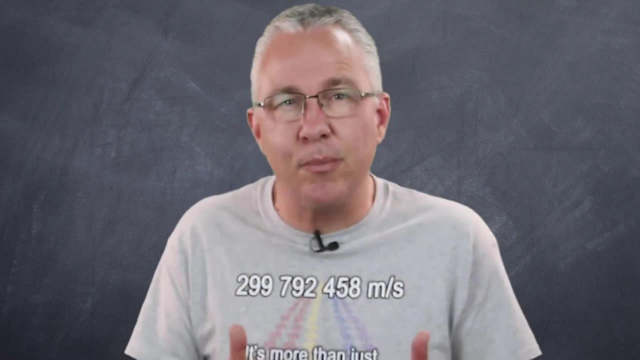 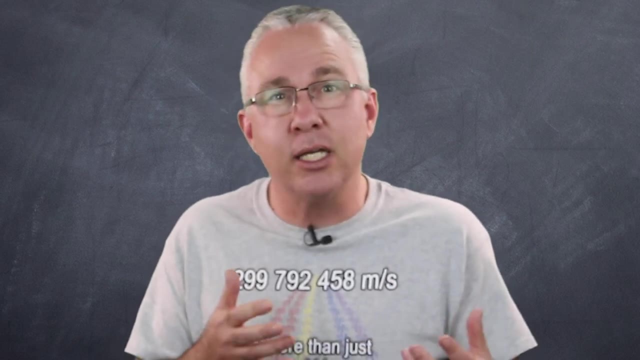 theoretical framework to explain it. Importantly, Compton came up with the presupposition that the collision between the x-rays and the electrons behaved in pretty much the same way that colliding billiards behave on a billiard table, That is, they behaved as particles, And the end result? 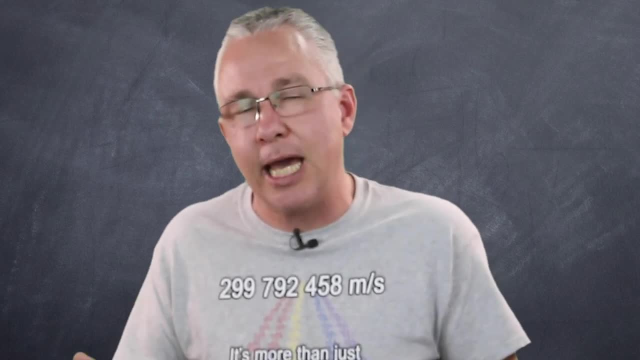 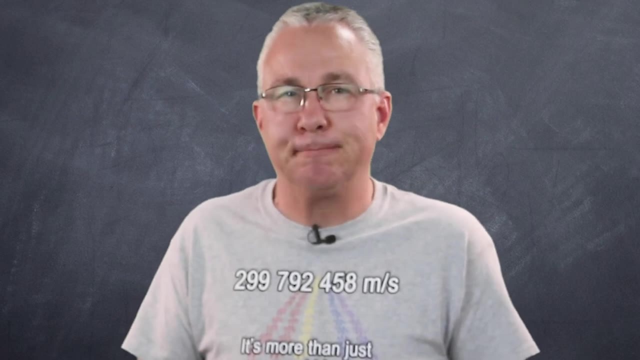 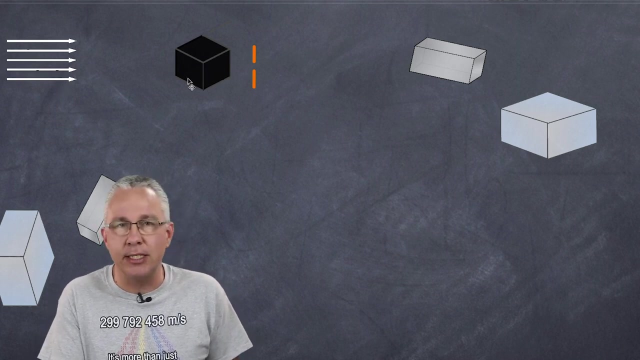 is what we now know as the Compton effect, Or Compton scattering, And it provided definitive evidence of the particle-like nature of light. Let's look at that more closely. So let's start by looking at Compton's experimental setup and see the results that he got. So here we have our incoming x-rays and they're going. 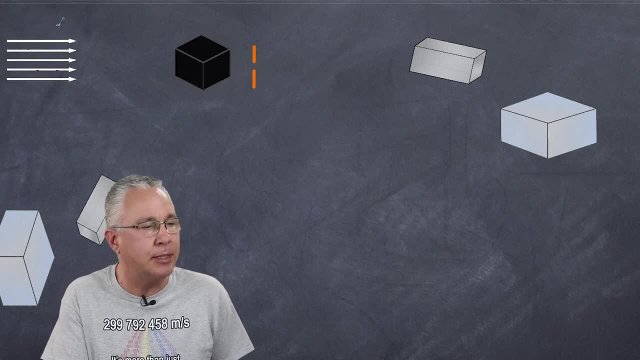 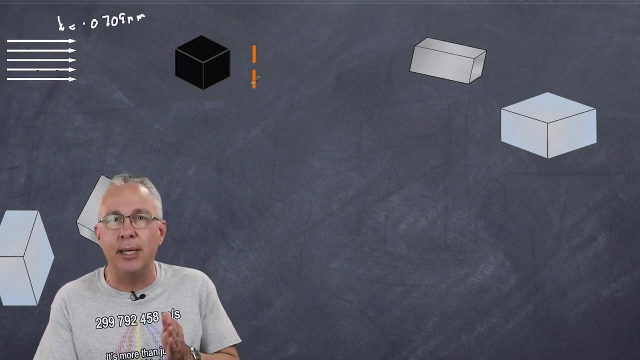 to be striking a graphite sample. Now, in the case of Compton's experiment, he had x-rays that were produced at a wavelength of 0.0709 nanometers. Then he set up a series of slits which, in essence, is a very similar to the one that we saw in the first experiment. So that is, you're able to isolate. 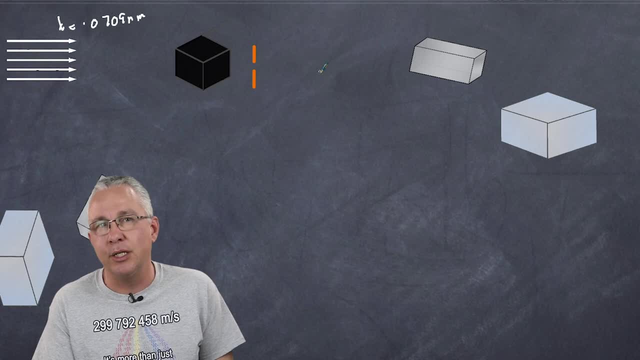 a particular beam of x-rays passing through, In this case because it's actually coming straight ahead. we're assuming that there is no scattering whatsoever Now. these then strike a calcite crystal and then hit what was referred to as an ionization chamber. I won't go specifically into. 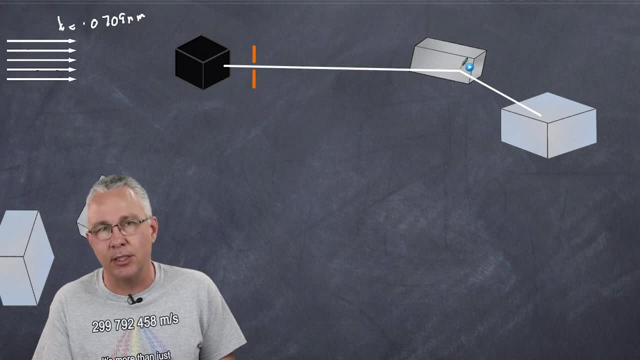 the physics here, but there is actually interference going on here that causes this deflection of the calcite chamber. This is referred to as a relationship related to Bragg's law, And then this shows him a strong signal. So, in essence, by placing this ionization chamber in the right, 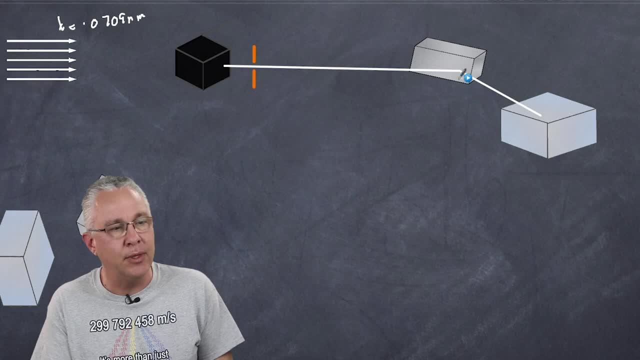 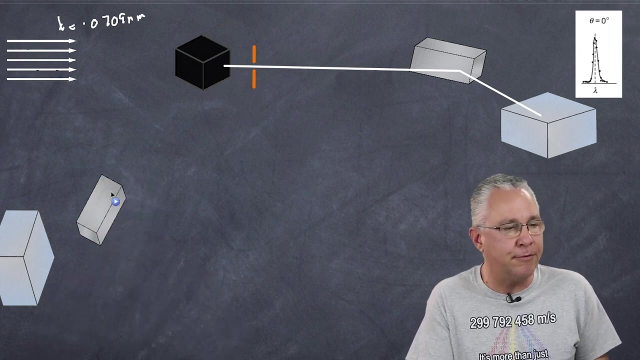 position, working out whether this deflection angle is here. he can then determine exactly what wavelength is coming in here, And the wavelength he's actually picking up here is actually our original wavelength of 0.0709 nanometers, But he noted that at a different. 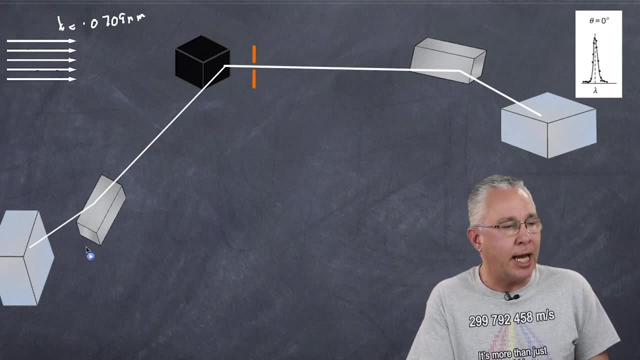 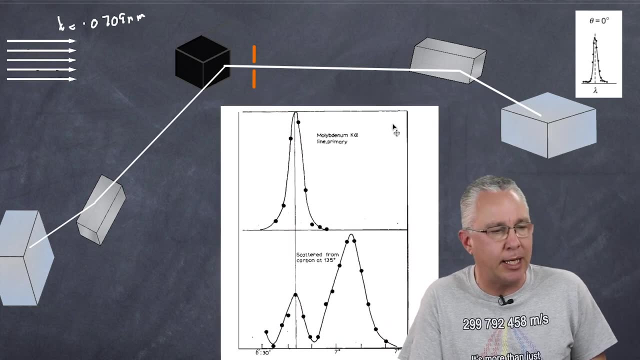 angle, in this case at 135 degrees, he actually ends up getting a result that is markedly different, And the result he ends up getting looks like this. Now let me explain it to you. This first peak is our original wavelength. Our original wavelength is appearing here, but you now get this. 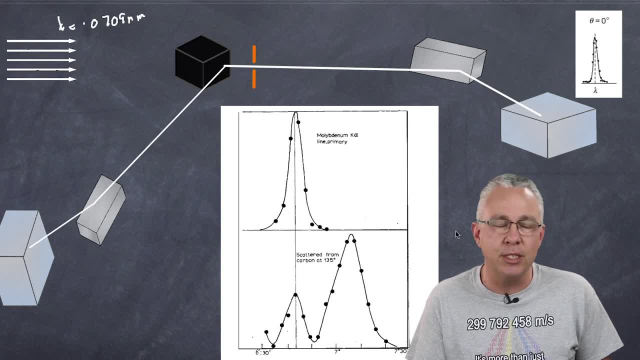 peak here further down. What he was able to show was that the majority of the x-rays that were coming and hitting this ionization chamber actually had a longer wavelength than the incoming wavelength that we have at 0.079 nanometers. Now I'll explain why we're. 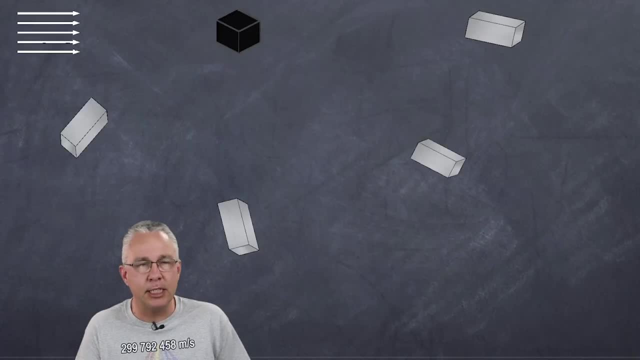 getting that little peak there in a moment. Then he set up the experiment to actually determine the relationship between the outgoing x-rays, that is, the angle at which they come out of the graphite box, and the amount of shift in terms of the wavelength away from the original So of 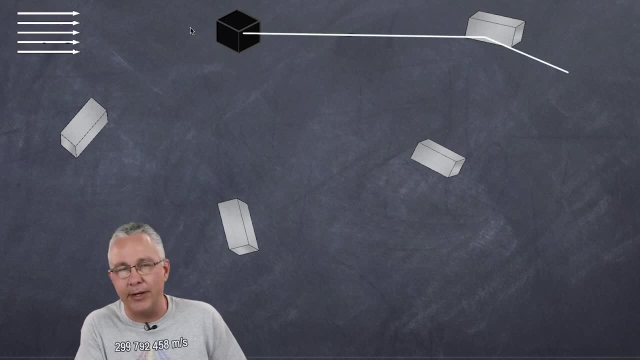 course, the first one is fairly straightforward. There's no scattering going of the substance here, and the results he got was of course our wavelength, which is lambda. But at first he's showing us that the angle of the x-ray coming down at 0.0270 nanometers is actually 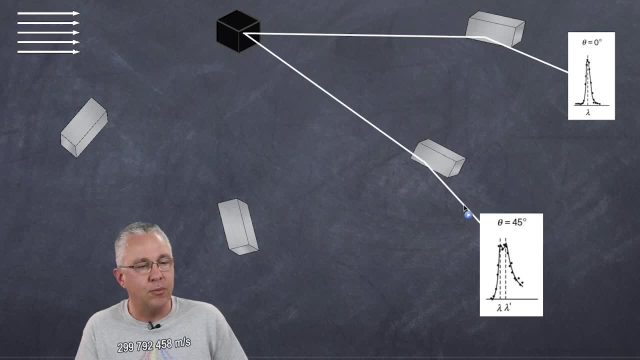 the amount of shift in terms of the wavelength away from the original. So of course, the first one is fairly straightforward- There's no scattering going of the substance here- and the results he got was of 45 degrees. what the result he got was this: you had certainly a small peak of his original wavelength. 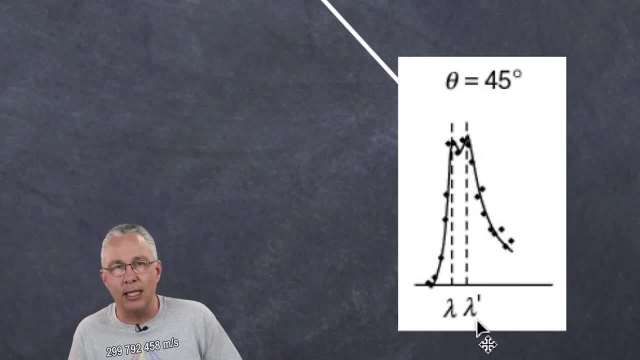 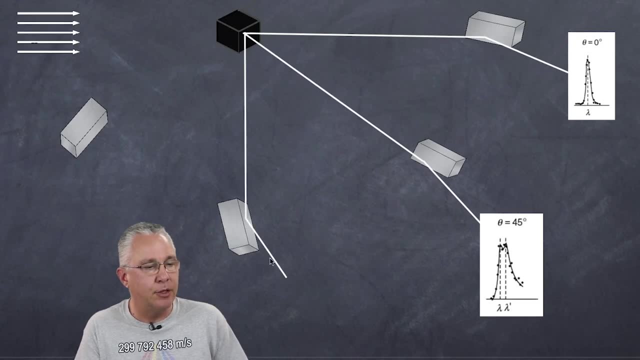 but we had a shift in the wavelength and we have here this lambda dash, which is a longer wavelength than the incoming wavelength that we had at the beginning. then at 90 degrees, the result was a greater shift. now notice here the difference between the lambda and the lambda dash. actually, 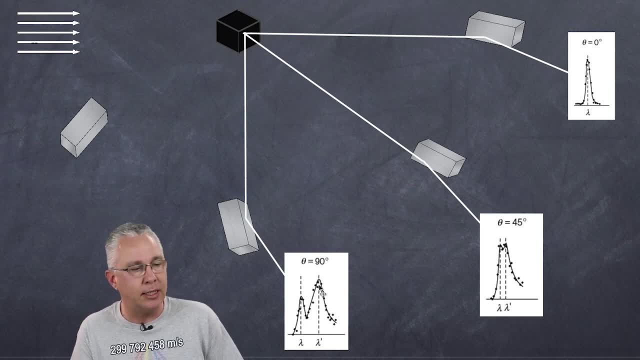 increases as our angle increases and you'll notice that the amount of x-rays that are of the longer wavelength is actually much bigger than the original size over here, and then finally, at 135, you get a much larger separation. here you can see that there's a much bigger increase in the 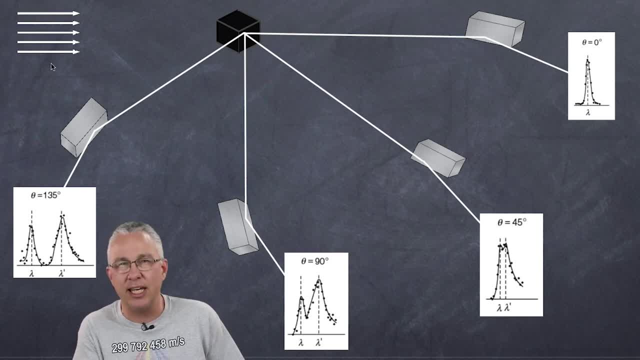 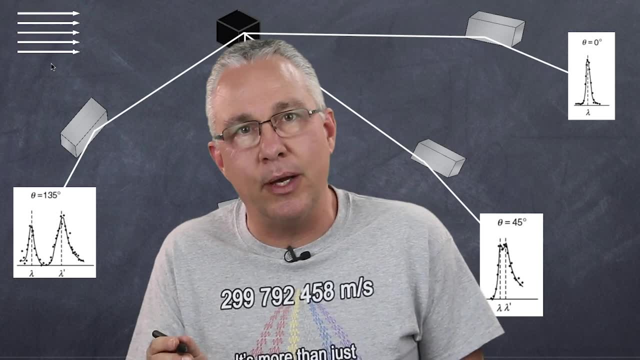 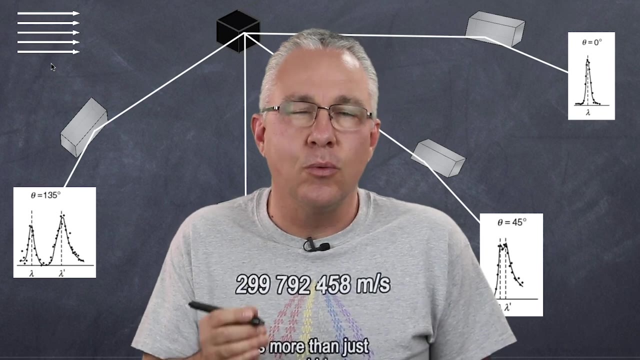 wavelength that we have from the incoming wavelength. in other words, the larger the angle of scattering, the bigger the difference between the incoming and outgoing wavelengths, and in fact, the outgoing wavelength is always longer, and what Compton wanted to do was to find a theoretical reason as to why this occurred. 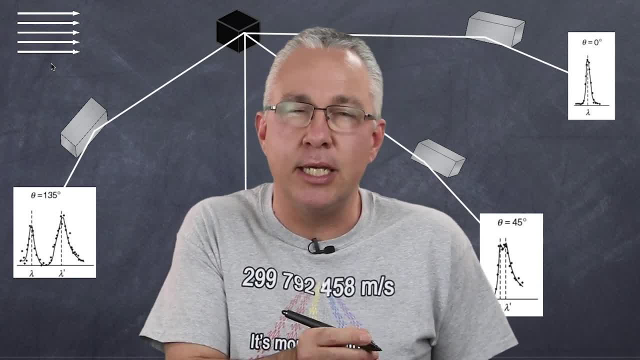 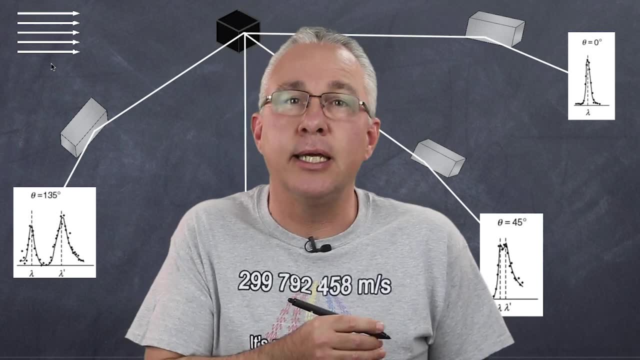 now, if this was talking about x-rays in the terms of electromagnetic radiation, in other words, energy as a continuous spectrum, then what you would expect is that the incoming wavelength would not change, no matter what the scattering is. but that's not what we get. we get a changing wavelength. 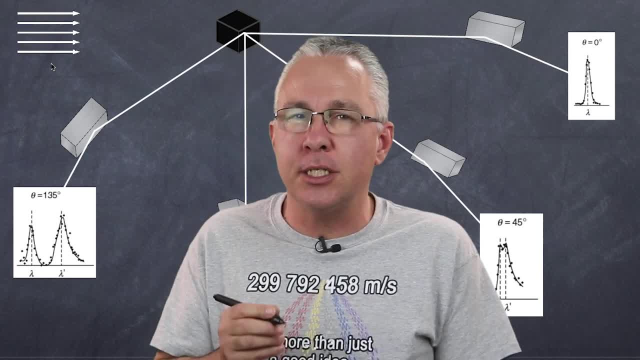 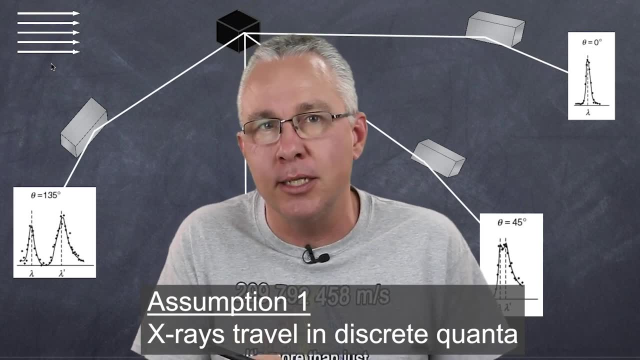 now, what Compton did was make a number of assumptions, and the first assumption he made was: how about we treat our x-rays not as a wave but as a particle, just like Einstein did when talking about light? because x-rays is a form of light, a form of electromagnetic radiation. 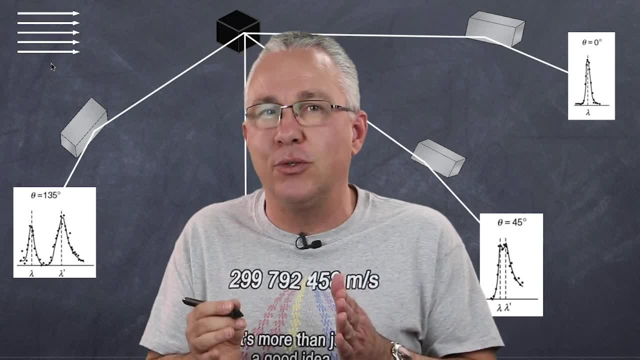 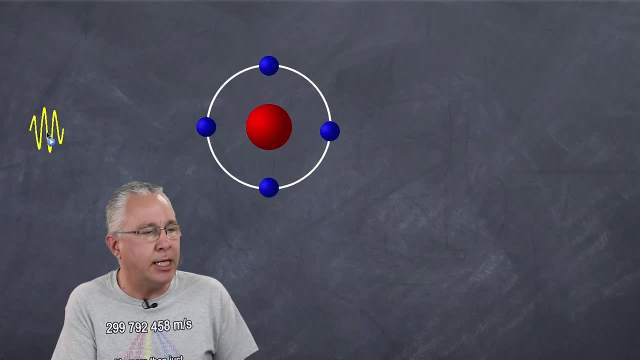 and that, too, should behave in terms of quanta, or discrete amounts, what we now know as photons, and so this is the interaction he started to theorize about. so here is our incoming photon of x-rays, or our incoming particle, as probably Compton referred it to me, and this particular 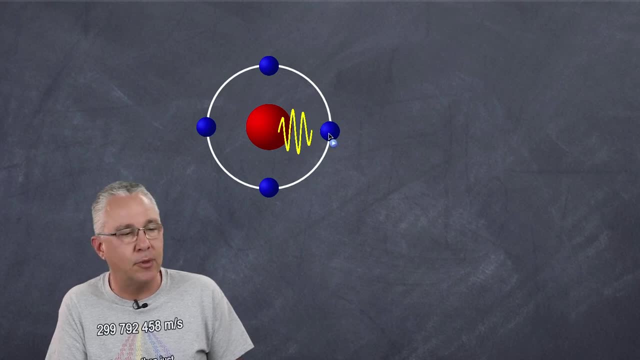 particle of x-rays would strike our outermost electron. now, how they might strike will determine which way the direction locker goes. the electron would glance off in a certain direction. in other words, the electron now has been given kinetic energy, but the end result is that we also get 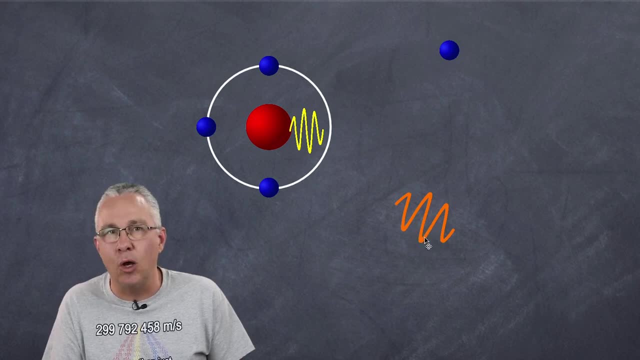 the release of another photon of x-rays, but in this case a longer wavelength, and the size of this wavelength is determined by the angle at which this deflection takes place. now, what about that original peak that was always appearing? well, if this particle of x-rays was 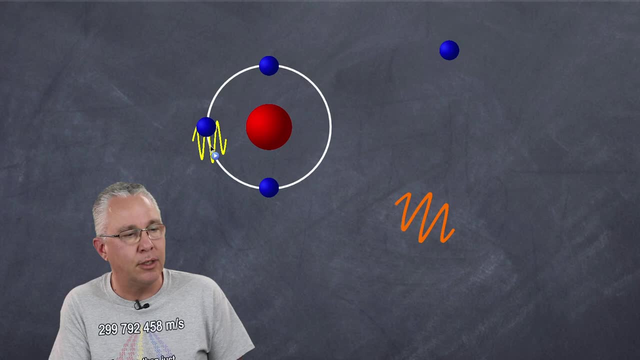 coming in and it didn't strike an outermost electron, but instead struck the nucleus, or struck the innermost electrons, then the electrons wouldn't escape, and so, in essence, the actual atom would vibrate at the same energy that it would have received the x-rays. so, in other words, what you get, 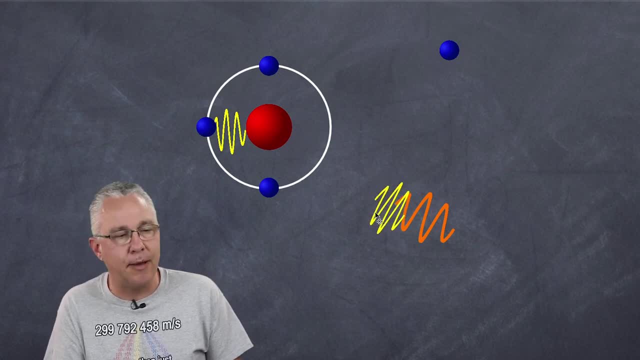 is another photon or another particle of x-rays coming out, but in this case it would be of the same wavelength. so, in essence, depending on the angle, you end up getting two here. now remember, this is not coming out of the one atom, this is coming out of the multitude of atoms that exist. 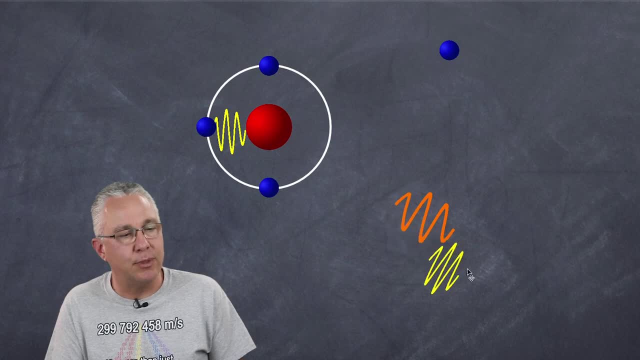 there. so some would travel here in this direction and then some, of course, will be from the deflection of these guys over here. but in essence you'd get two peaks as a result. but the beauty is is that the wavelength here is actually the same as the incoming wavelength. so now let's have a look at 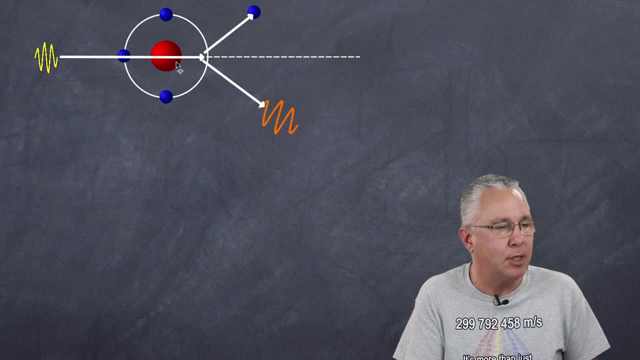 this in terms of a little bit more what compton did mathematically. so here's our photon coming in and of course, it's striking off and as a result, we get this particular angle. now there are two angles here, and the angle i'm going to refer to in this case is phi. now there is also the angle. 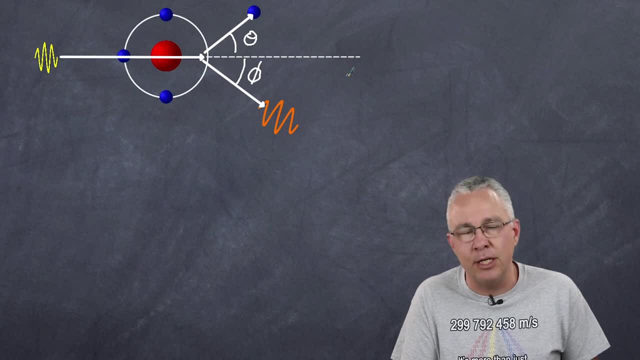 theta, which is the scattering angle of the electron. now, compton wasn't interested in the electron, he was interested in looking at the photon. remember what he's trying to do. what is the relationship between wavelength here- wavelength here l dash- and phi, which is the angle right here? 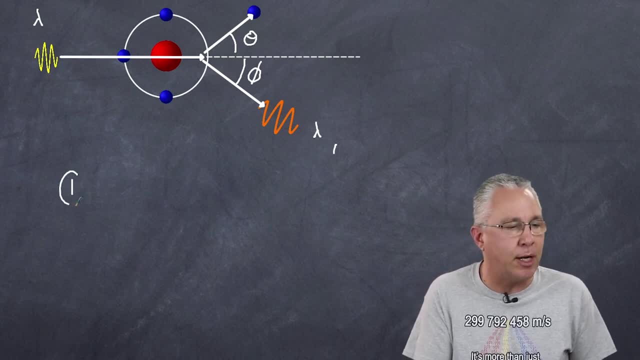 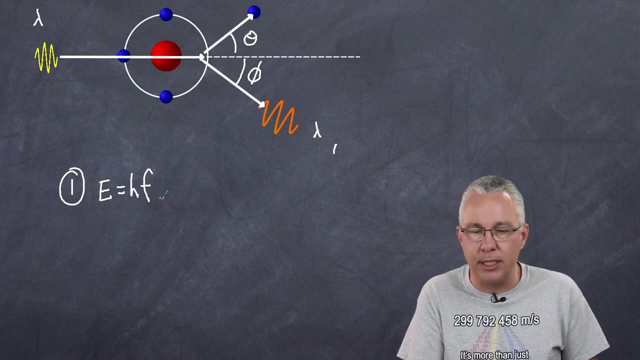 and, as i said, he made a number of assumptions, and assumption number one, which i've already stated, is that basically, these are acting as particles. that means that they have an energy that is related to h- f, in other words, e is equal to x, constant multiplied by the frequency, and that 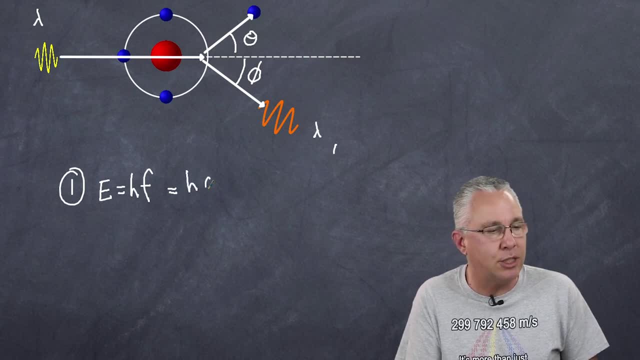 of course. if i then substitute the frequency, we get hc over lambda. so that's our first assumption: they are acting like particles. now, the second assumption that he made was that, basically, the energy of any particular component is equal to the relativistic energy formula, that is, e squared is equal to p squared, c squared. 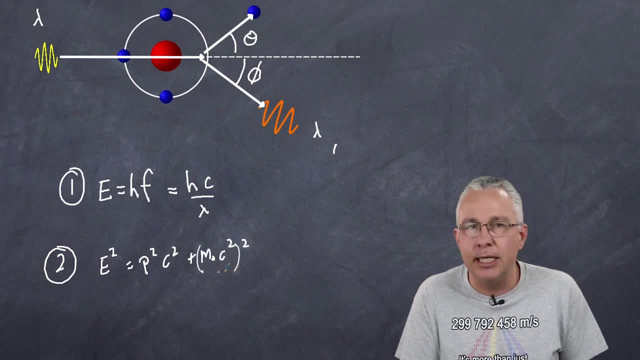 plus m naught c squared. squared is our famous e equals mc squared formula. that is, we call the rest energy of a particle, but if we then apply this to our particle of X-rays, it has no mass, and so, as a result, what you end up getting is that E squared is equal to P squared, C squared, and that, of course, 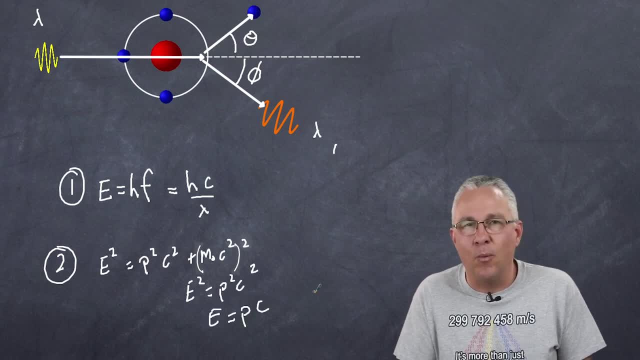 means E is equal to PC, and what this tells you straight away is that our photon, our particle of X-rays, has momentum, and that's critical. what you end up getting is that the momentum is equal to the energy that we have up here, of course, divided by the speed of light, and that, of course, is equal to HF over C. 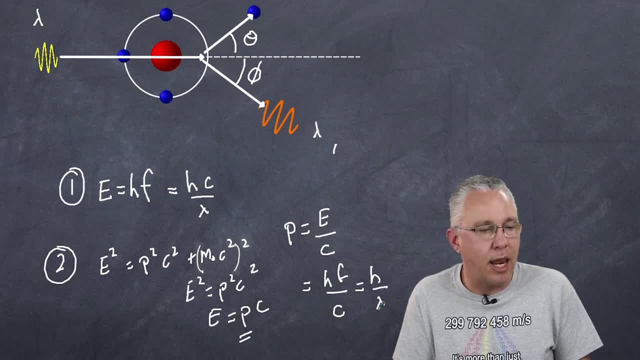 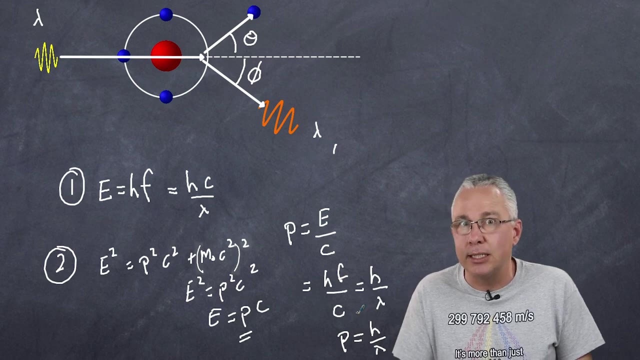 and of course that is ends up being H over lambda. Now we have that particle wave duality, that is, the momentum is equal to H over lambda and that it words anything that has a wavelength there automatically means it has a momentum, even though it hasn't got any mass. So that's a second assumption, and 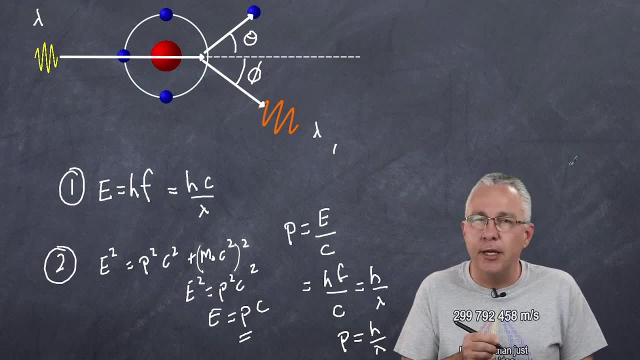 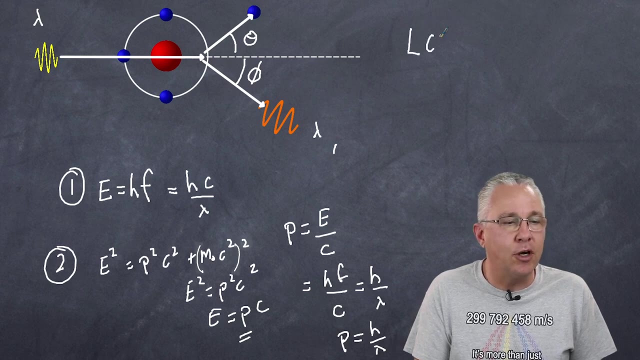 now we get to the third assumption. The third and crucial assumption: If my particle of X-rays has energy and my particle of X-rays has momentum, and clearly electron also has energy momentum after the interaction, then the law of conservation of momentum has to remain true and the law of the 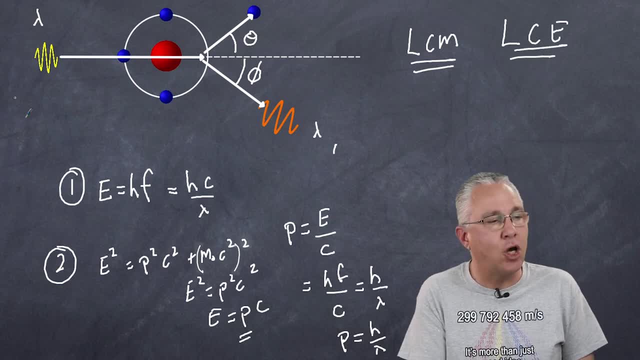 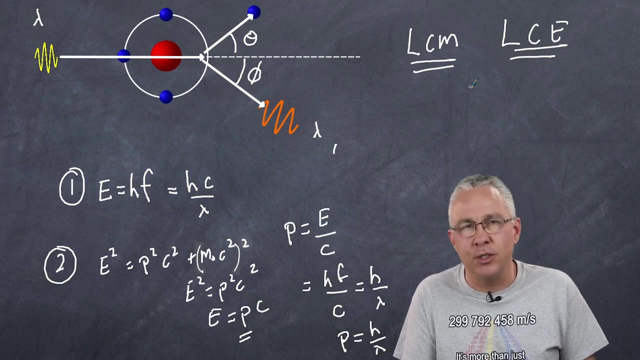 conservation of energy have to be true, That is, the total energy before the collision has to equal to the total energy after the collision. The total momentum before the collision equals the total momentum after the collision. and so he then set out, using those two particular laws- and you probably know them already- to determine: 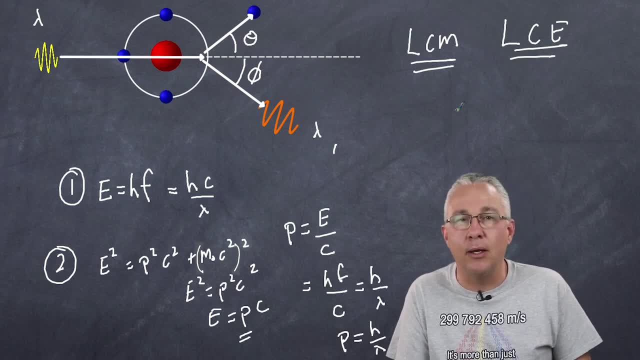 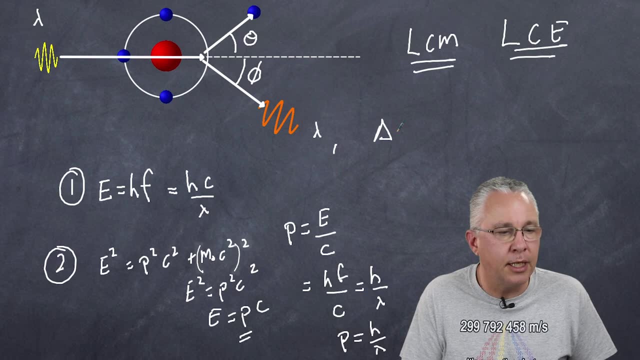 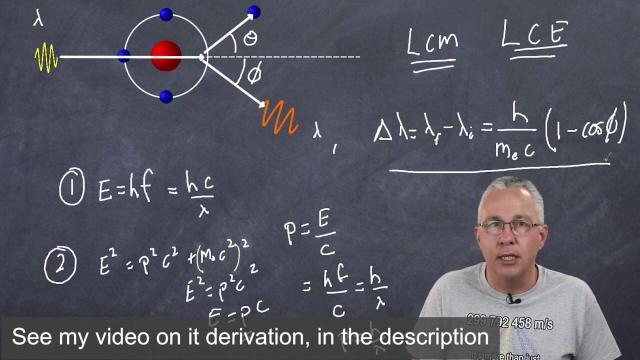 the relationship between the ingoing and outgoing wavelengths and the angle at which the scattering takes place, and he comes up with this formula: The difference in wavelength, which is basically my outgoing wavelength minus my ingoing wavelength, is equal to H over lambda MEC, outside of 1 minus the cosine of our angle phi. Now this explains Compton. 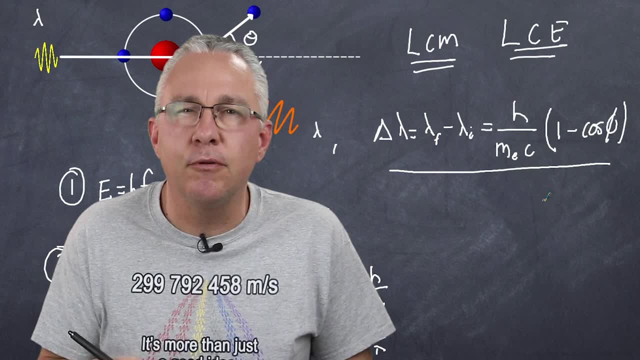 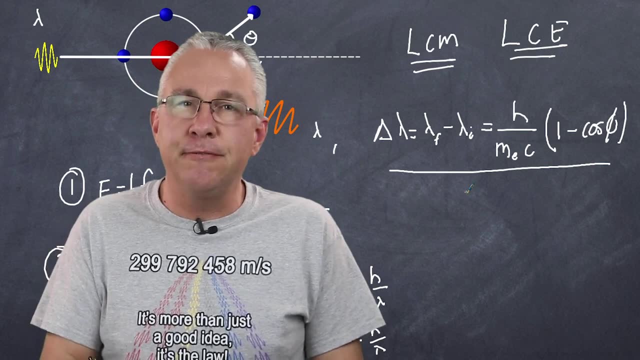 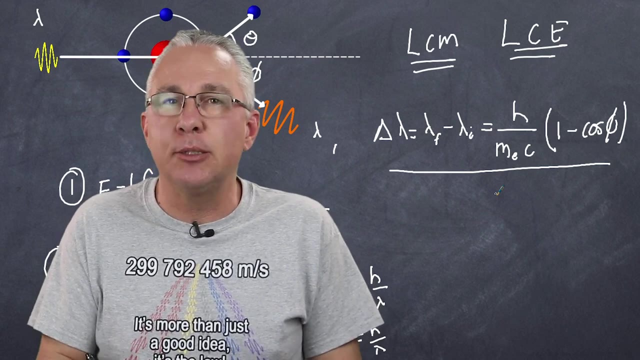 scattering or the Compton effect. Compton himself remarked how consistent the mathematics fit with the experimental evidence. So he definitively verified here: by treating X-rays as quanta or as particles he could explain the scattering of X-rays coming off substances. This was definitive evidence. 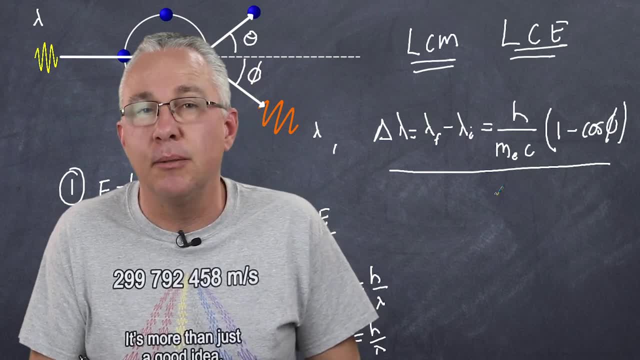 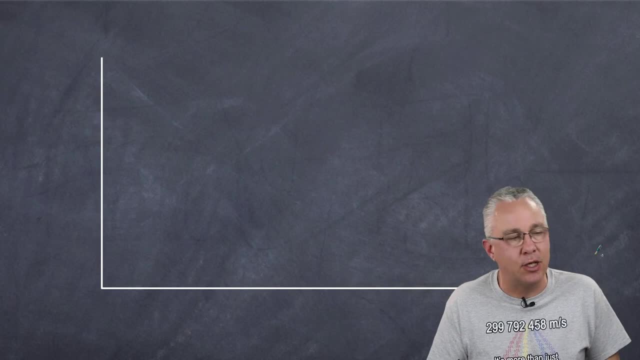 to support the idea. and in this case, light, in terms of X-rays at least, behaves as particles. Finally, what I want to do is look at some graphical analysis of that. So let's say, on our y-axis we put our change in our wavelength, then on our x-axis we put in our angle. here and remember the formula is: 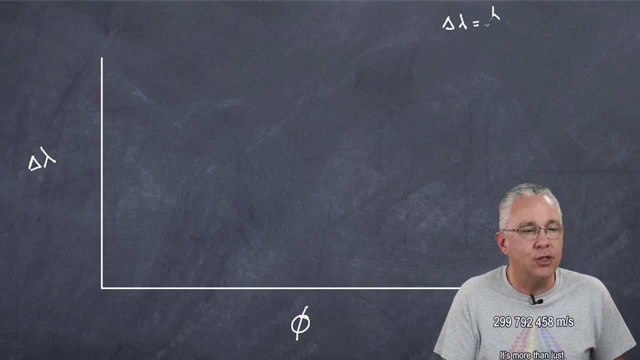 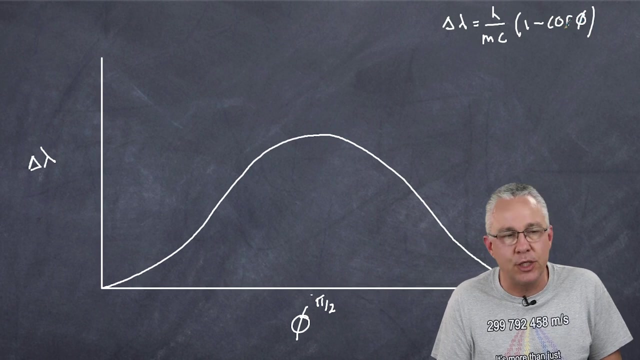 that the delta of lambda is equal to H over MC outside of 1 minus the cosine of phi, And if you graph that, you get a graph that looks like this: At an angle of 0, the cos of 0 is 1 and therefore we get no change in wavelengths At the 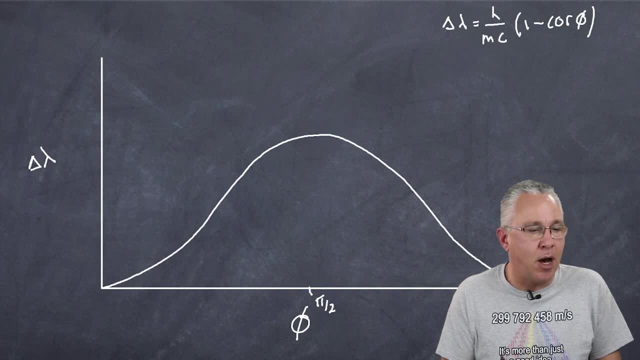 angle here, which is our in these terms of radians, angle of pi over 2, and cosine phi is equal to 0. And so you end up getting the change being H over MC, and that here is the value of H over MC, and this term here is referred to as the Compton wavelength.